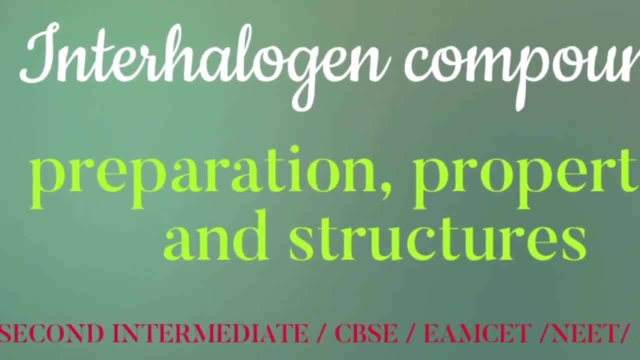 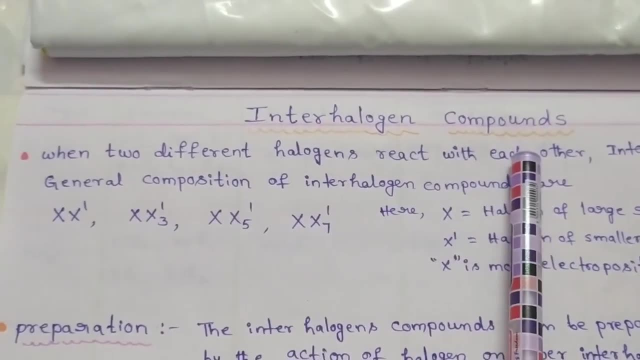 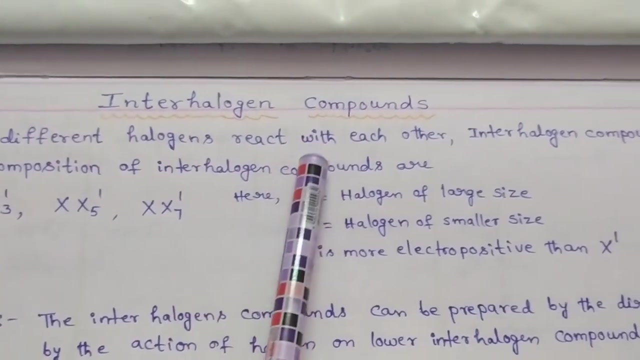 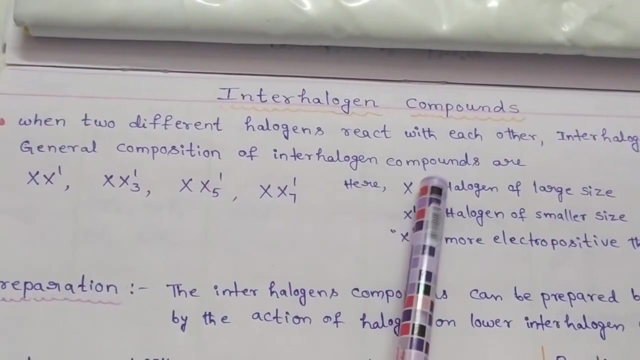 Hi students, today we discuss interhalogen compounds. The definition of interhalogen compounds is: when two different halogens reacts with each other, interhalogen compounds are formed. The general composition of interhalogen compounds are X- X' type X- X3' type X- X3'. 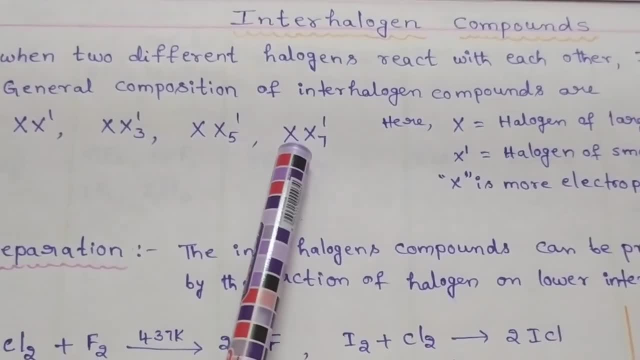 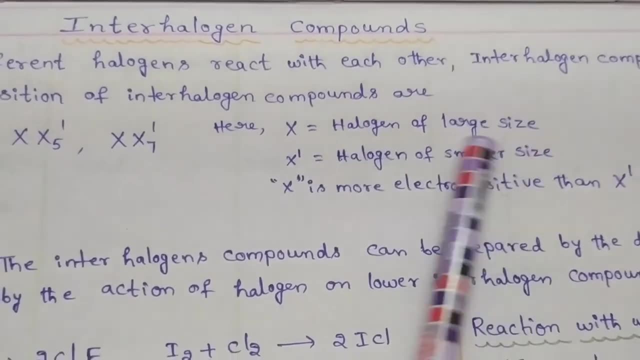 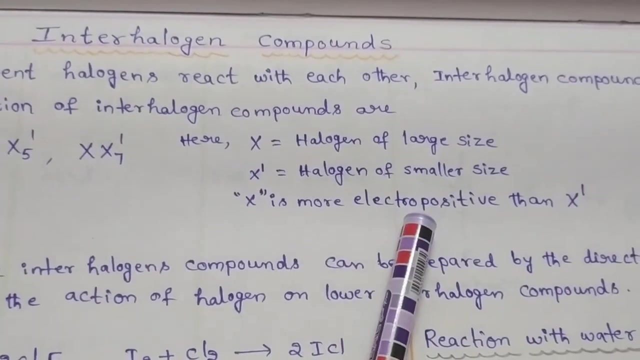 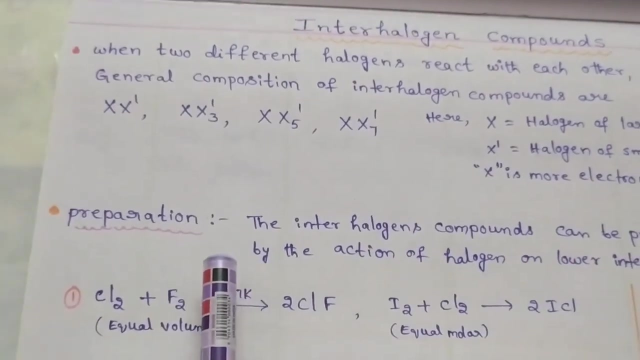 X, X5' type X, X7' type of compounds. Here X means halogens of larger in size, X' means halogens of smaller in size. Here X is more electropositive in nature than X' type of halogen compound. Now we discuss the preparation of interhalogen compounds. The interhalogen 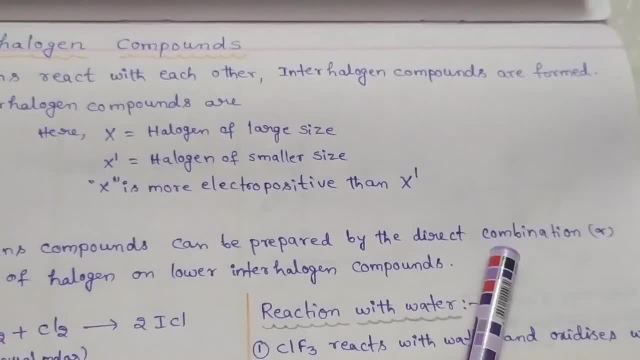 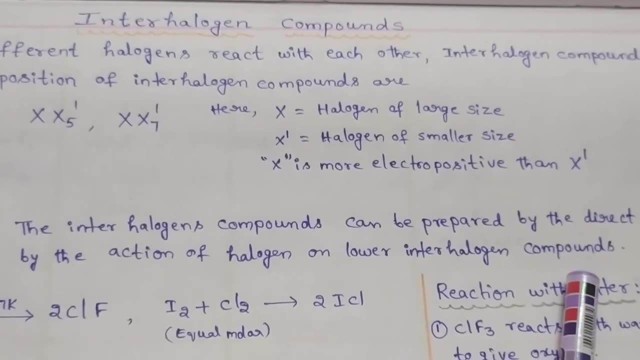 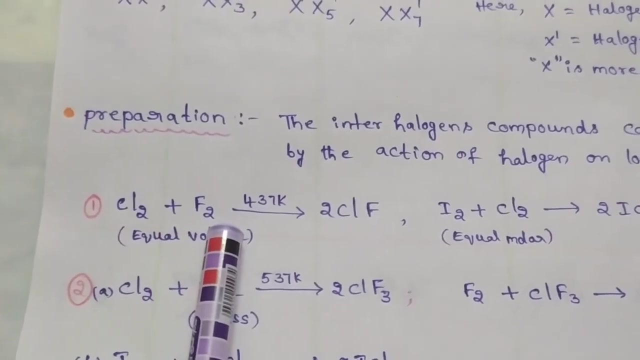 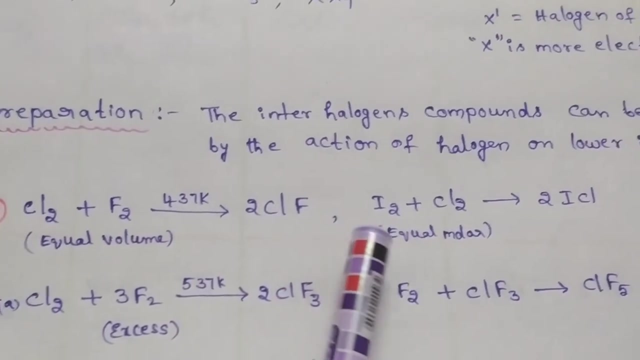 compounds can be prepared by the direct combination or by the action of halogen on lower interhalogen compounds, For example, when we can take equal volume of chlorine and fluorine molecules and they are heated up to 437 Kelvin. temperature form: chlorine monofluoride or equal molar. 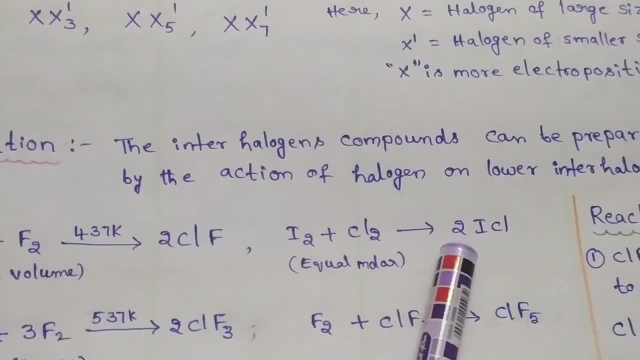 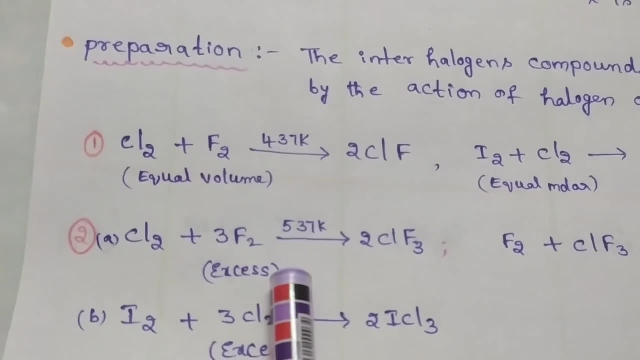 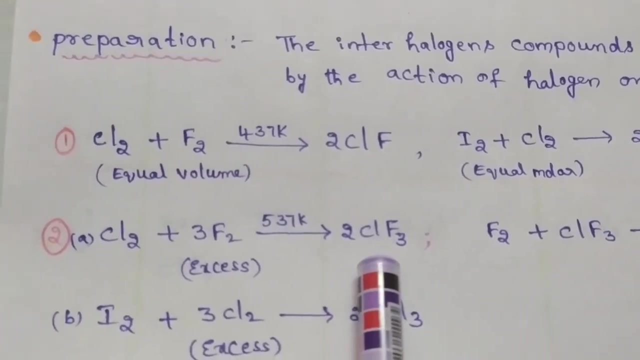 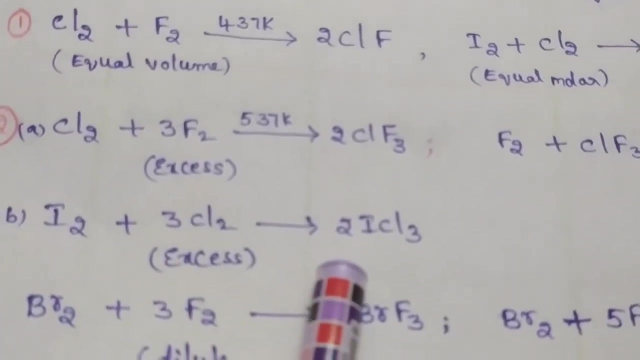 compositions of iodine and chlorine are reacted together. When chlorine is reacted with excess of chlorine molecule Unheated up to 537 Kelvin. temperature form chlorine trifluoride. When iodine is reacted with excess of chlorine: form iodine trifluoride. When bromine is reacted with dilute fluorine: form bromine trifluoride. I form Iodine tripofluoride. I form iodine triphluoride when bromine turns from bloating to diluting. I form Iodine trapyl purposes. I form acontecer, assuming that all the monochlorides 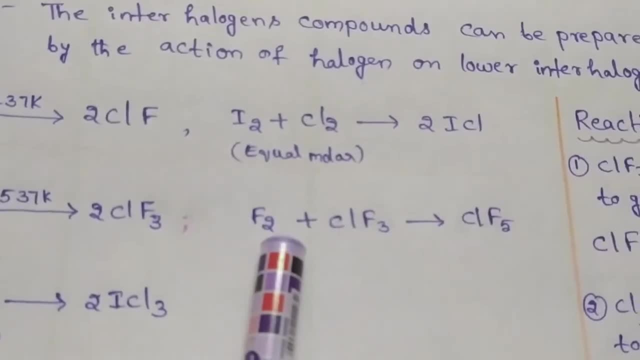 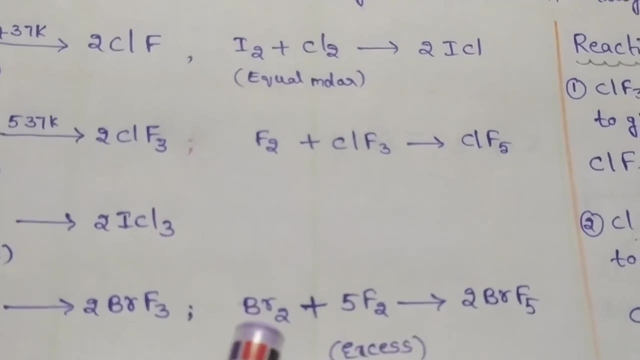 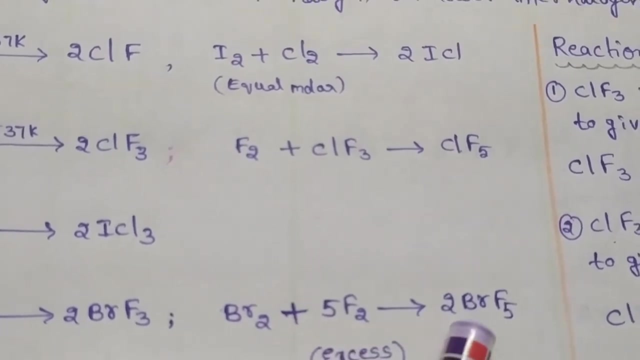 are reacting withsch underestimate. Ok. when chlorine react with the excess of chlorine molecule: Bromine trifluoride molecule. When fluorine is reacted with chlorine trifluoride molecule. form chlorine pentafluoride. When bromine is reacted with excess of fluorine, here we can take 1 is to 5 ratio form: bromine pentafluoride molecule. 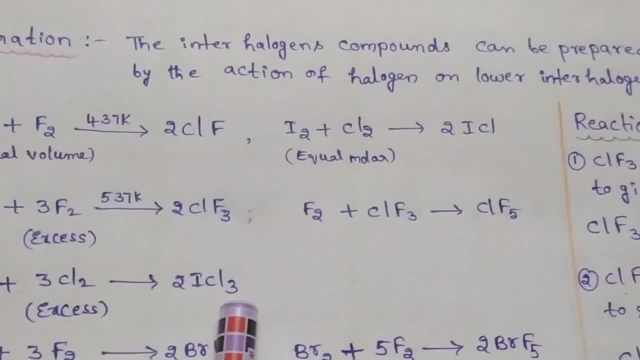 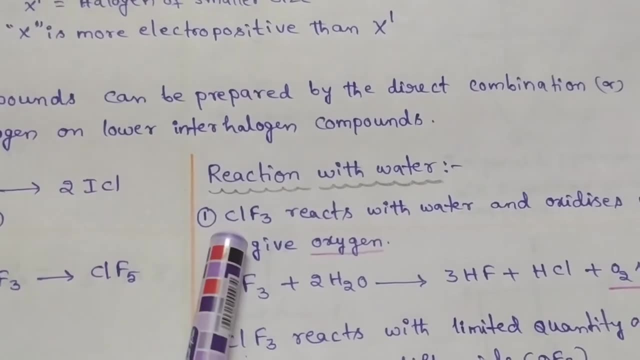 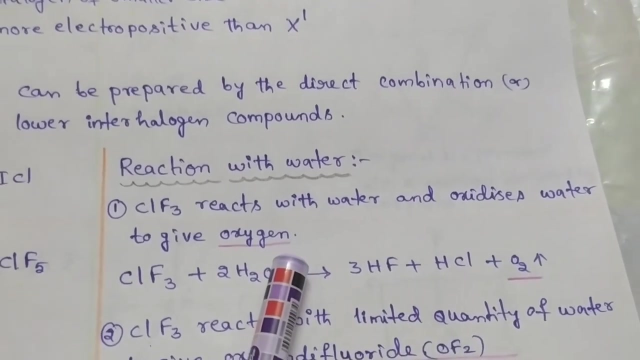 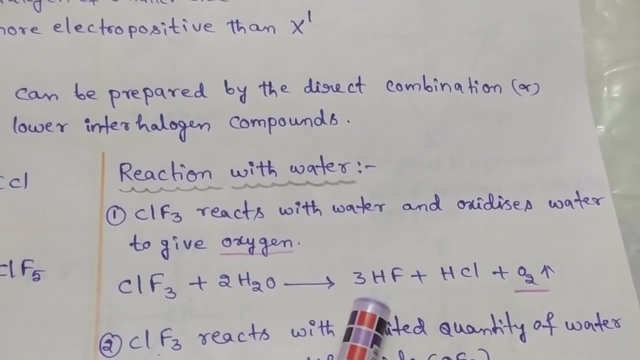 These are the preparation methods of interhalogen compounds. Now we discuss the reaction of chlorine trifluoride molecule with water. When chlorine trifluoride reacted with water and oxidizes water to give oxygen, For example, when chlorine trifluoride is reacted with 2 moles of water, molecule form, hydrofluoric acid, hydrochloric acid and oxygen gas is released. 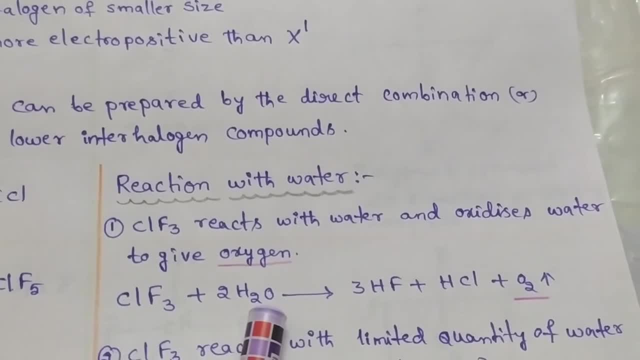 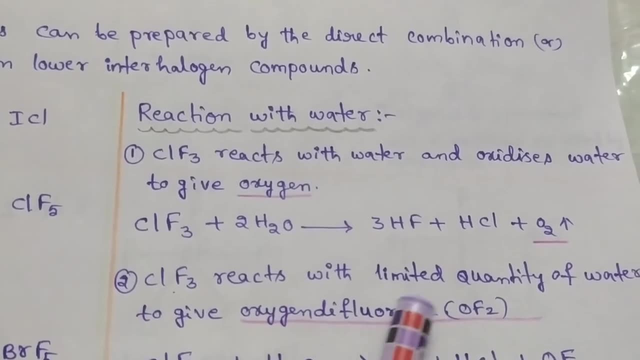 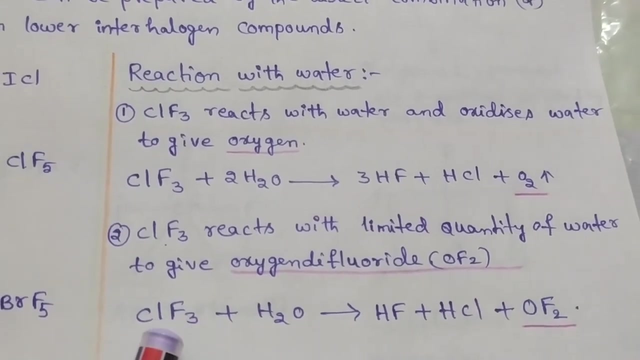 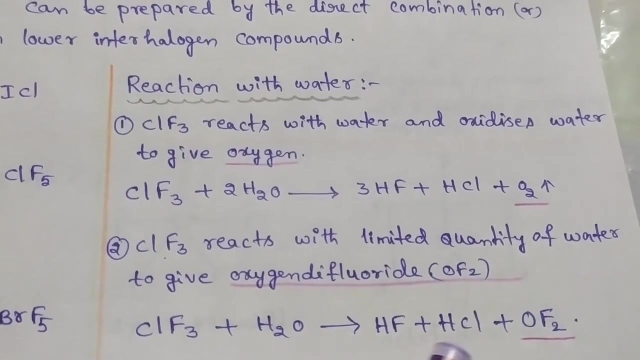 That means here this water molecule Is oxidized as oxygen molecule. When chlorine trifluoride reacts with limited quantity of water to give oxygen difluoride molecule, The reaction is chlorine trifluoride is reacted with 1 mole of water. molecule form hydrofluoric acid, hydrochloric acid and oxygen difluoride molecule is formed. 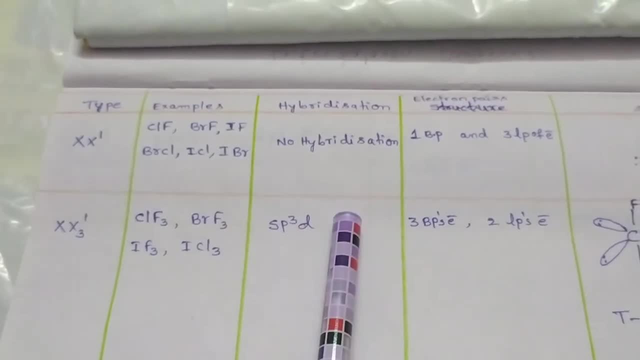 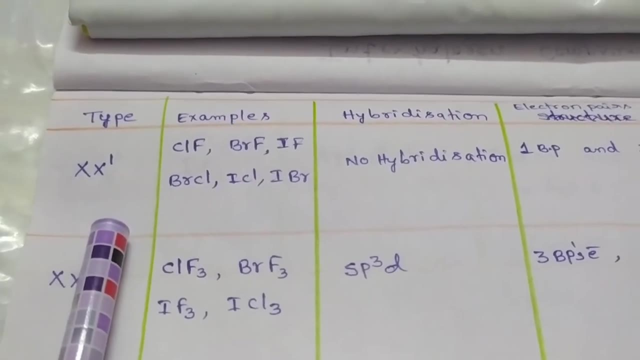 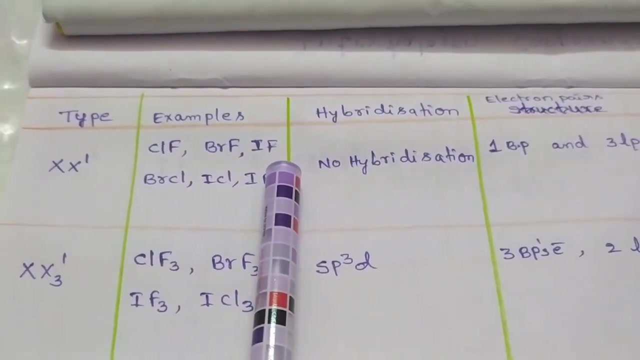 Now we discuss the hybridization and structures of interhalogen compounds. First, XX-type of molecules. Examples are: chlorine monofluoride, bromine monofluoride, iodine monofluoride, bromine monochloride, iodine monochloride, iodine monobromide. 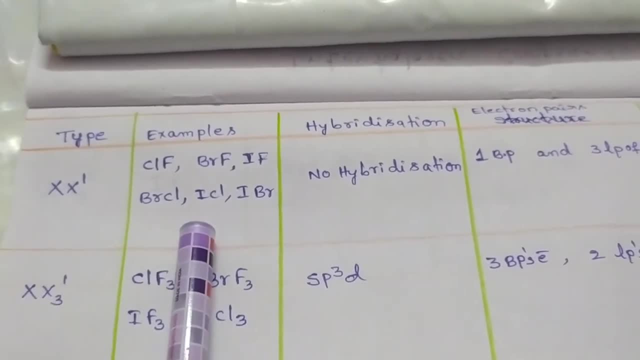 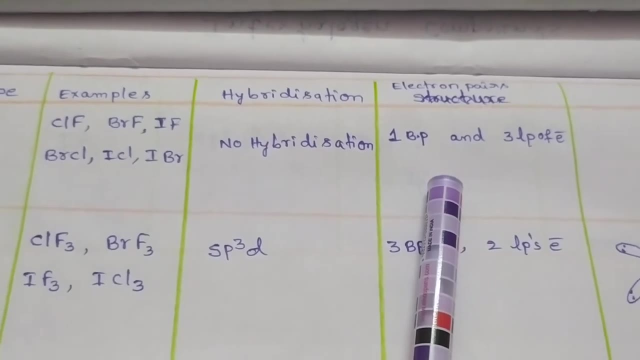 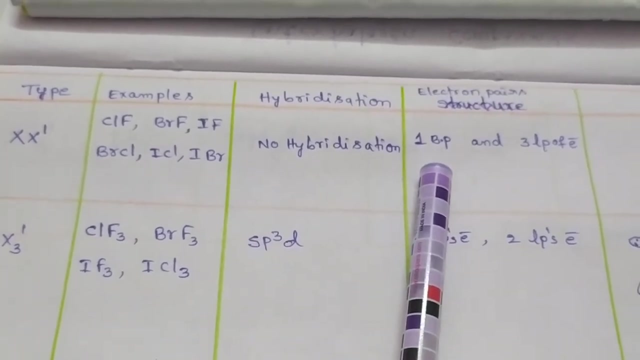 These are XX-type of molecules. Hybridization: There is no hybridization. There is no hybridization. Electron pairs: According to Valenci shell electron pair repulsion theory, XX-type of compounds are having 1 bond pair of electron and 3 lone pairs of electrons. 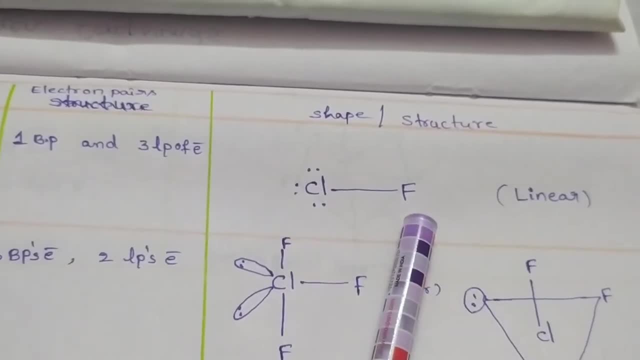 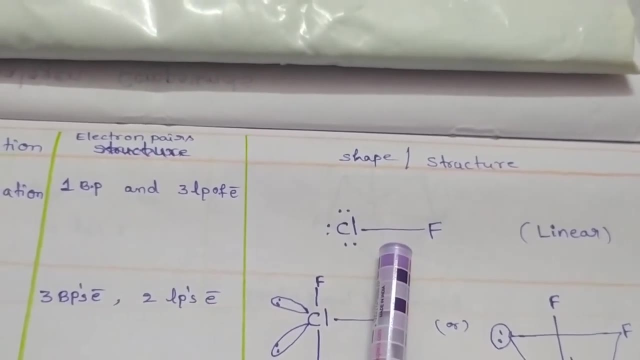 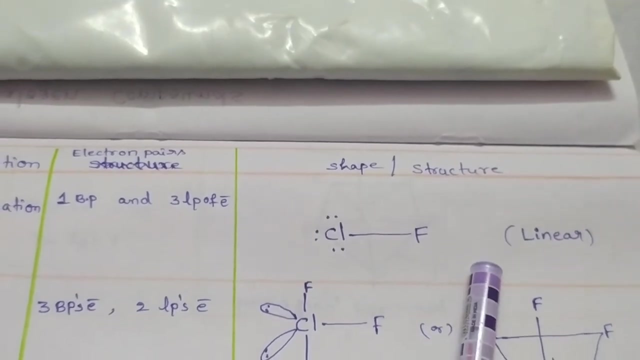 For example chlorine monofluoride. Here the chlorine is the central atom. This chlorine having 1 bond pair with fluorine atom And 3 lone pair of electrons are there. This is a linear shape in structure. Now we discuss XX-type of molecules. 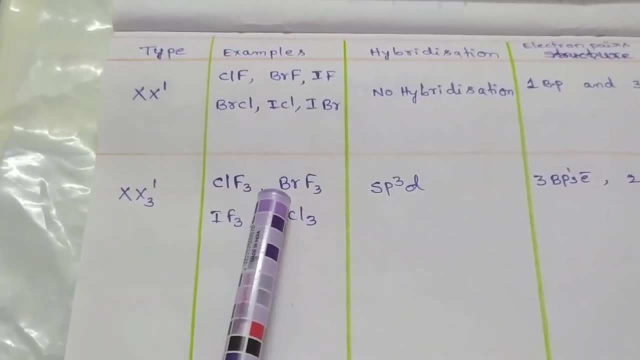 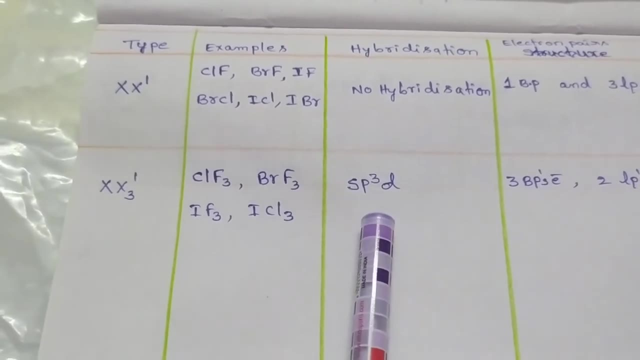 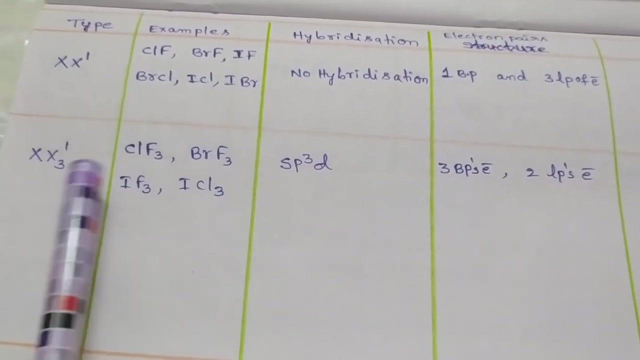 Examples are: chlorine trifluoride, bromine trifluoride iodine trifluoride iodine trichloride. The hybridization is SP-3D hybridization. According to Valenci shell electron pair repulsion theory, XX-type of compounds are having: 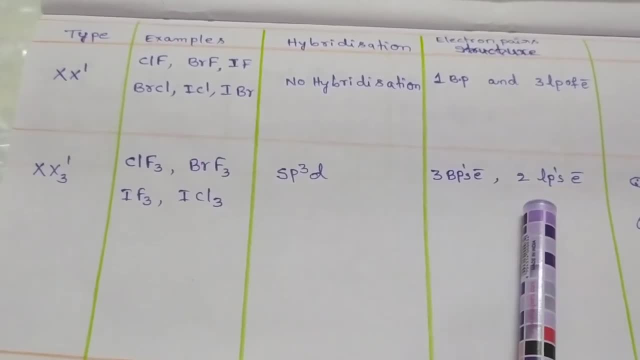 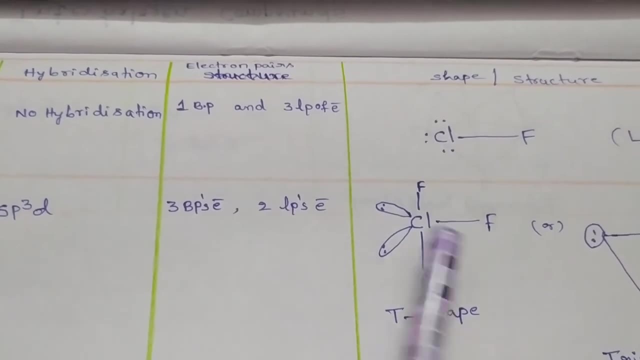 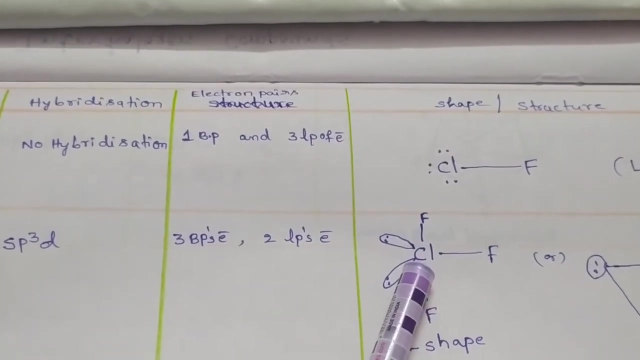 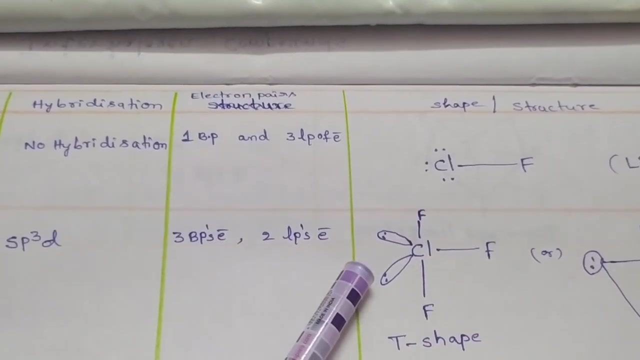 having three bond pairs of electrons and two lone pairs of electrons. For example, we can take chlorine trifluoride molecule. In chlorine trifluoride molecule, chlorine is the central atom. This chlorine bonded with three fluorine atoms and have three bond pairs of electrons and two lone pairs of. 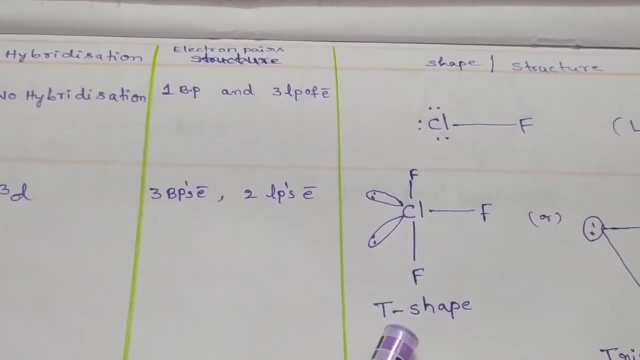 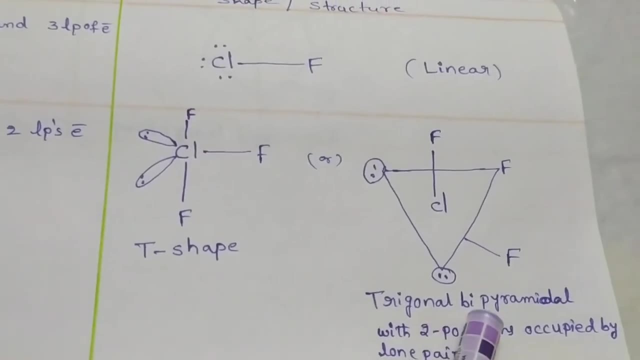 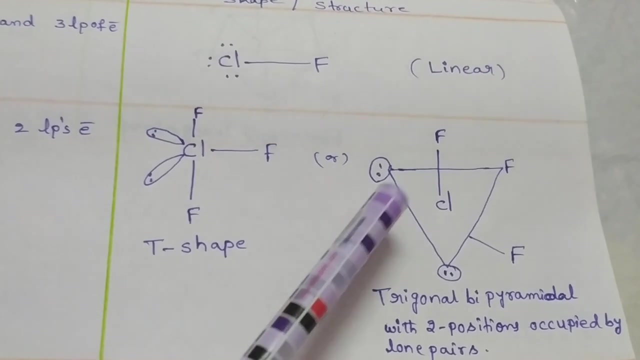 electrons are there. This is a T shape of structure. Another possible structure of chlorine trifluoride is trigonal bipyramidal shape, with two positions occupied by lone pair of electrons. This is the trigonal bipyramidal shape of structure of chlorine trifluoride molecule, with two lone pairs of 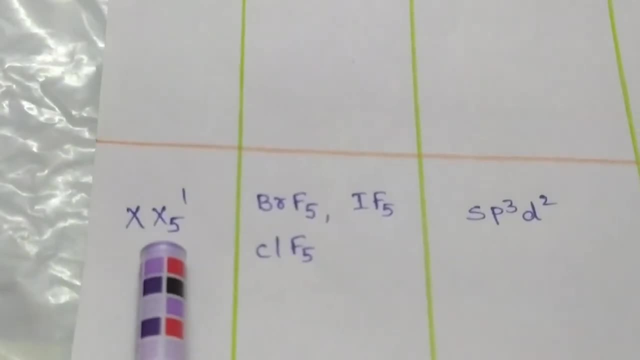 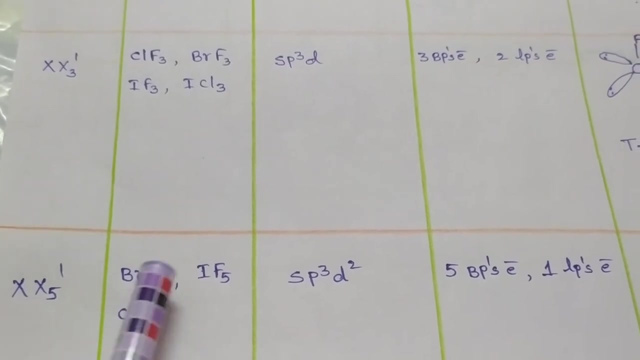 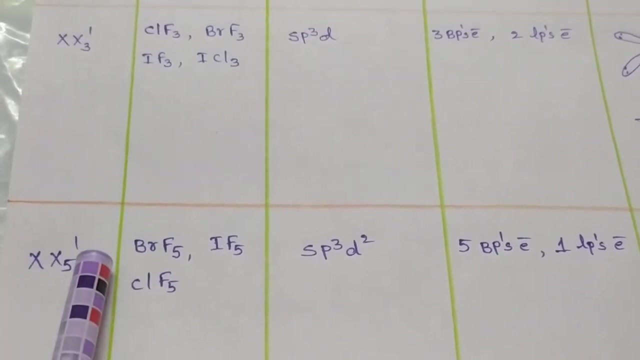 electrons. Now we discuss X5- type of compounds. Examples are bromine pentafluoride, iodine pentafluoride, chlorine pentafluoride. X5- type of compounds having sp3d2 hybridization. 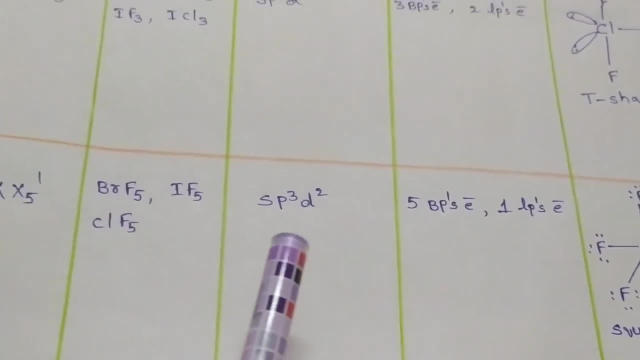 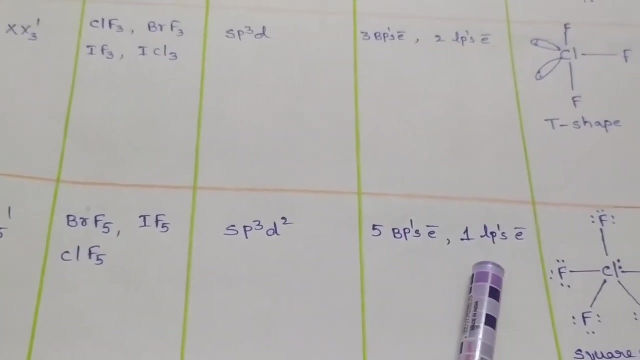 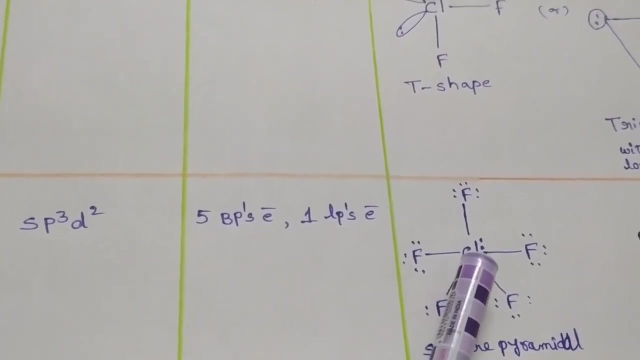 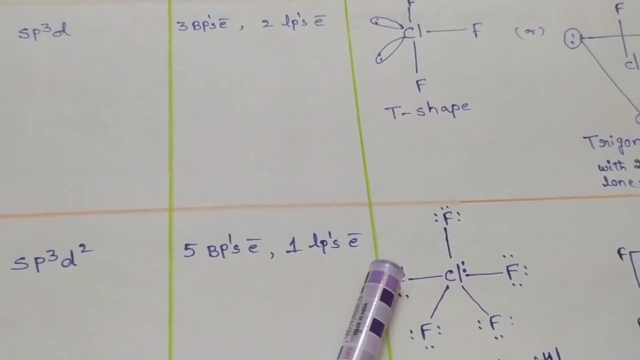 According to Valenci shell electron pair repulsion theory, X5- type of compounds having five bond pairs of electrons and one lone pair of electrons, For example chlorine pentafluoride molecule. Here the chlorine is the central atom. This chlorine formed five bond pairs of electrons, with five 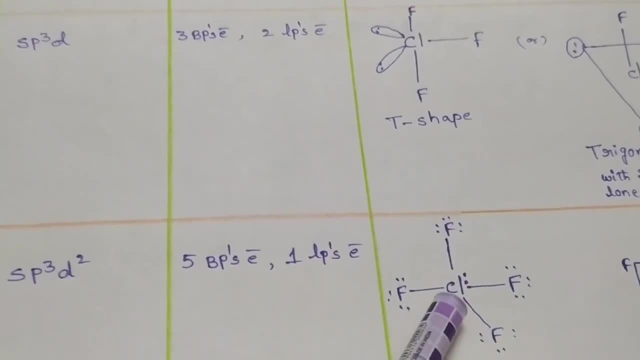 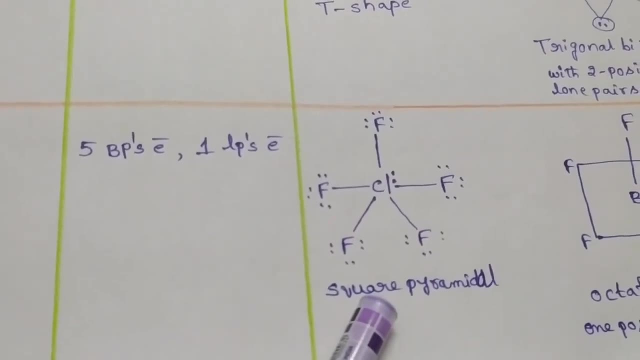 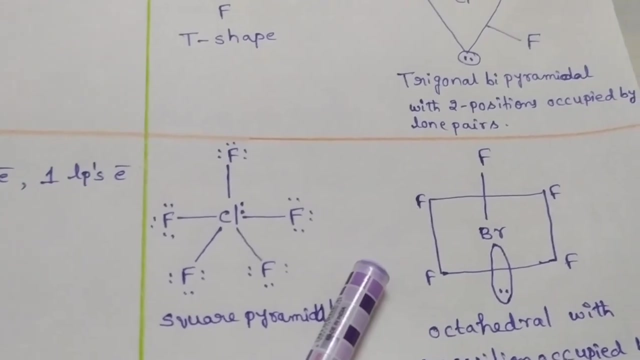 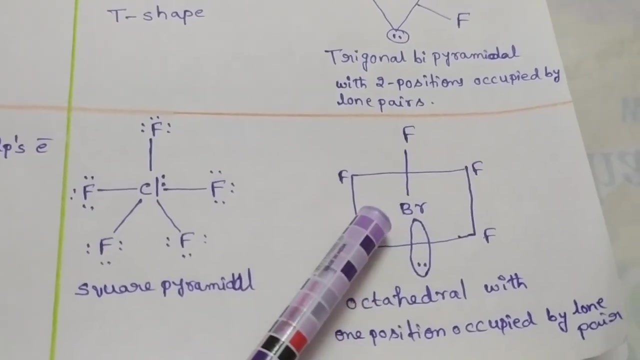 different fluorine atoms and the central chlorine atom containing one lone pair of electron. This is a square, pyramidal shape of structure. Another possible structure of chlorine trifluoride molecule is the strat들. This is a structure of X- X5' type of molecule is bromine pentafluoride, Here the bromine pentafluoride. 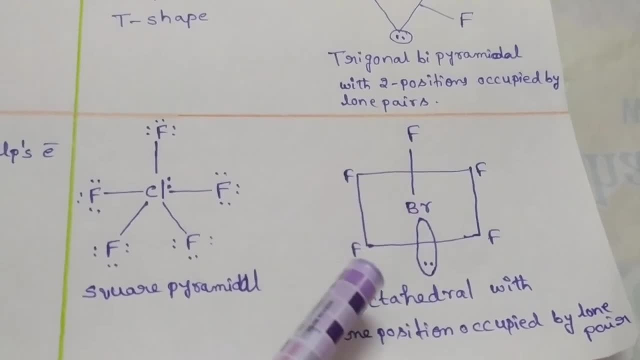 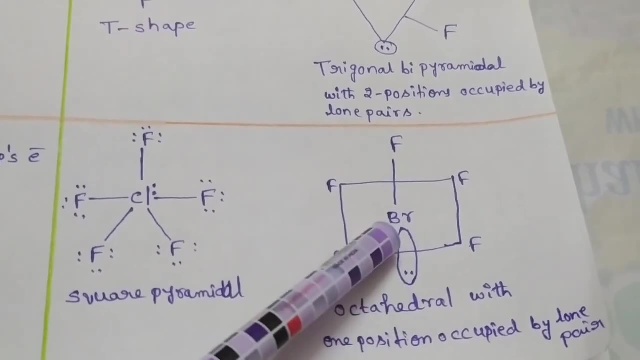 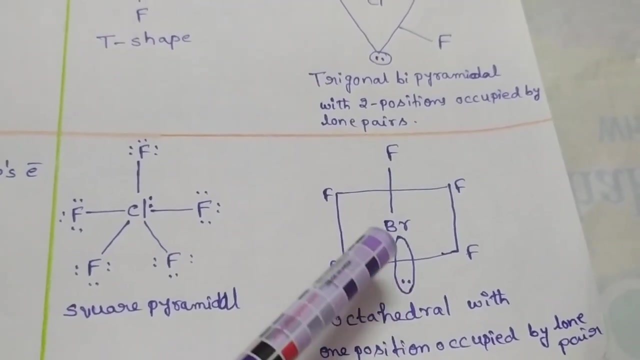 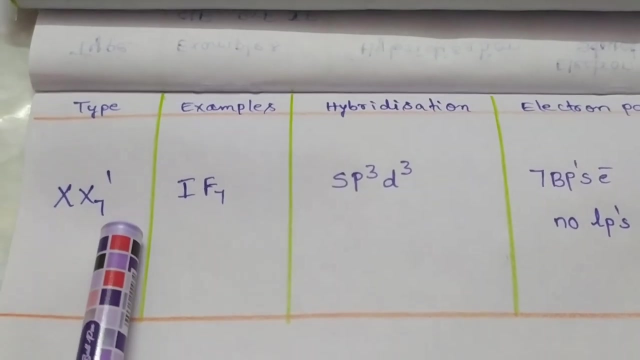 bromine is the central atom. This exhibit octahedral shape of structure with one lone pair of electron. here This is the octahedral shape of structure with lone pair of electron. This is the structure of bromine pentafluoride molecule. Now we discuss the X- X7' type of